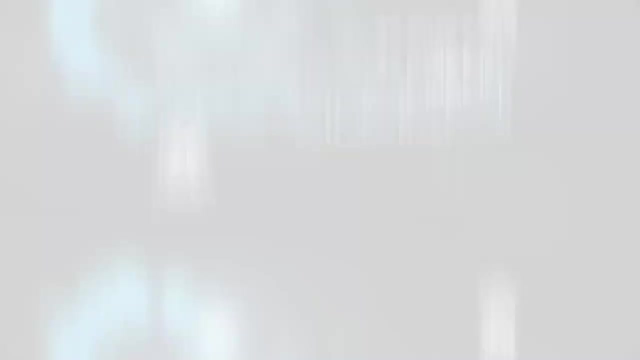 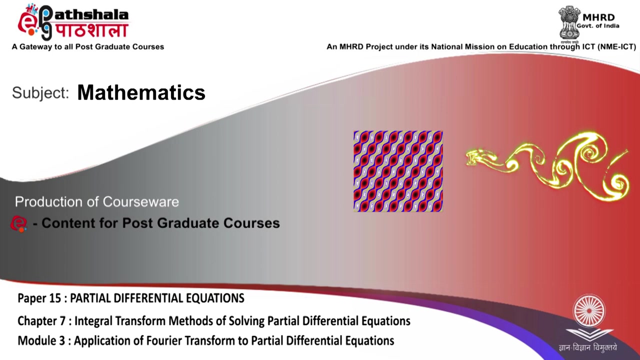 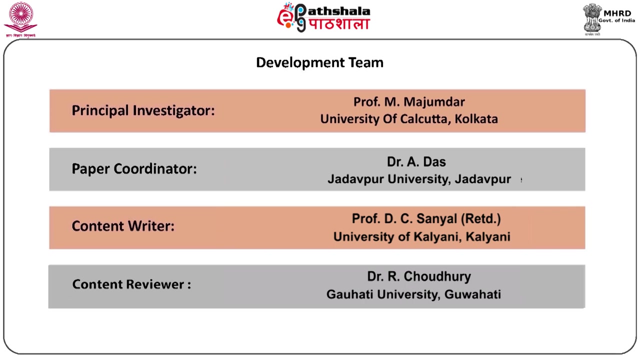 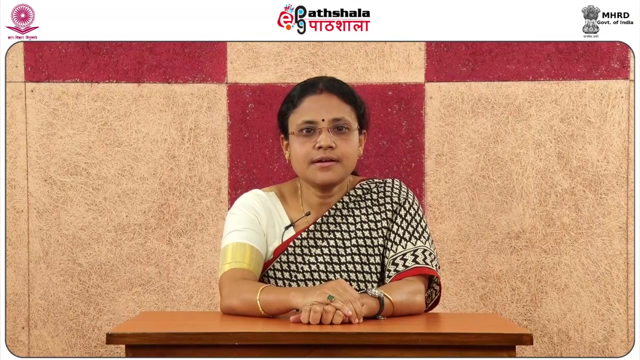 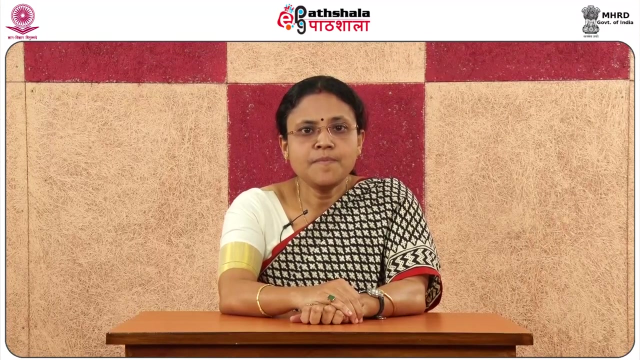 Now I am going to start module 3 of chapter 7.. In this module I want to mention that Fourier transform is a general transformation. Many other transformation, like Laplace transformation, Malin transformation, Henkel transformation, can be defined in terms of complex Fourier transformation. 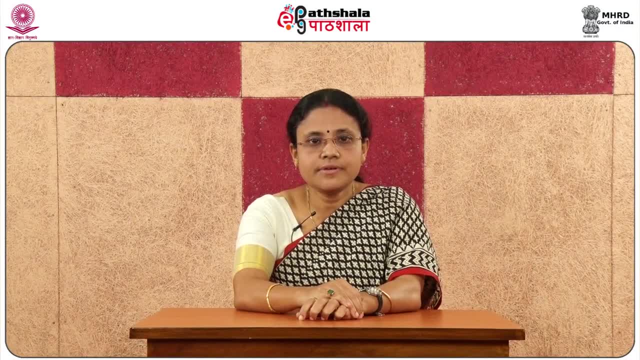 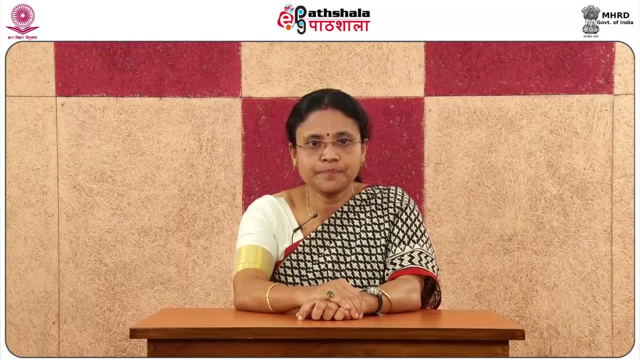 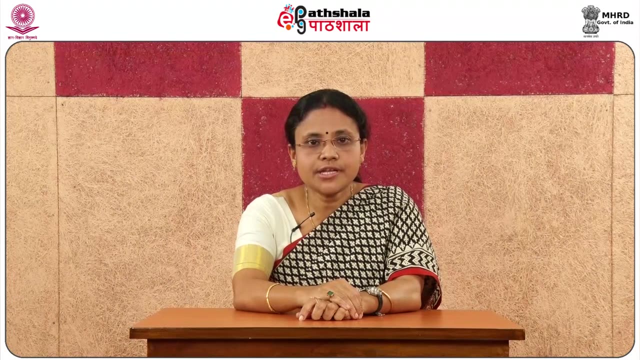 Therefore it is relevant to discuss about the application of Fourier transform to partial differential equation. In this module we shall solve the Laplace equation, heat equation and wave equation using Fourier transformation method. Now we are going to slideshow. First we shall start with Laplace equation. 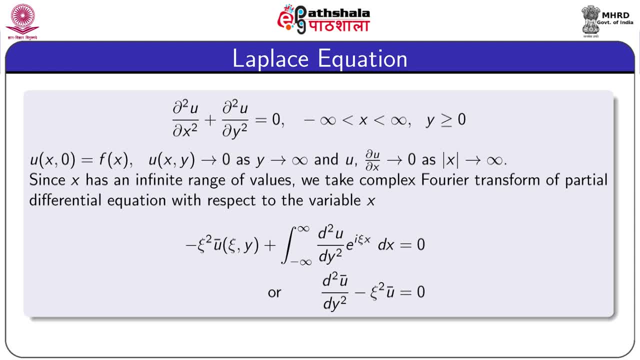 The Laplace equation in Cartesian coordinate system is given by del 2? u del x square plus del 2? u del y square equals to 0. Here we have considered infinite range for x and y is greater equals to 0.. We have also the initial condition for u: u at t equals to 0 is equal. 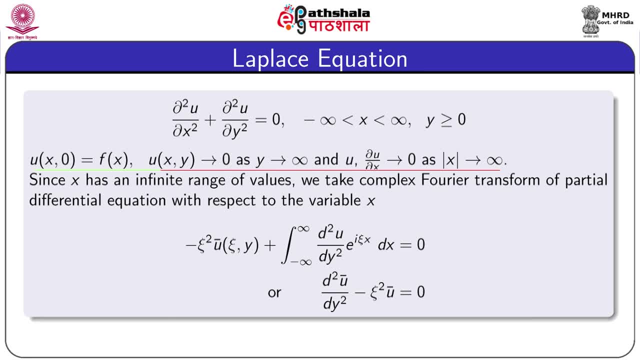 to f x. We also have u x. y tends to 0 as y tends to infinity. We have u del u del x. both quantity tends to 0 as mod x tends to infinity. Since x has infinite range of values, we take complex. 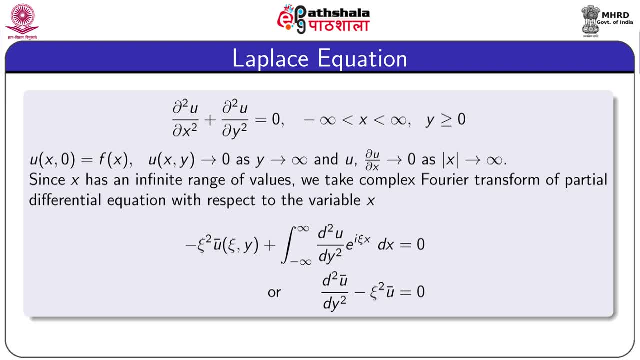 Fourier transform of the given equation with respect to variable x. Therefore, in the first dimension of doing Laplace equation we get: So we multiply the Laplace equation with e to the power, i, xi, x, and then integrate over x from minus infinity to plus infinity. The first term gives minus xi, square u bar xi. 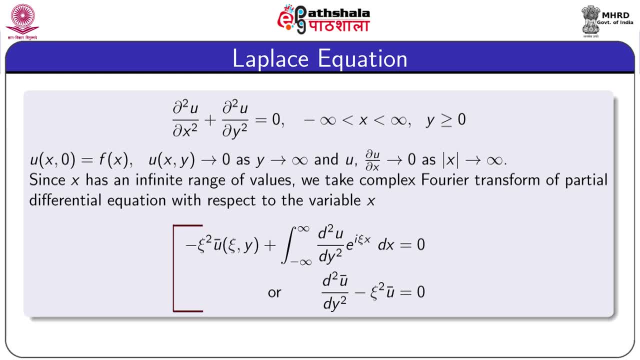 y, and the second term is plus integration. minus infinity to plus infinity: d, 2, u, d, y, square e to the power, x, i, xi, x, dx equals to 0.. Here xi is the transformed variable and the dependent variable, or u is transformed to the function u bar. So u bar is now function of xi and y. If you look at, 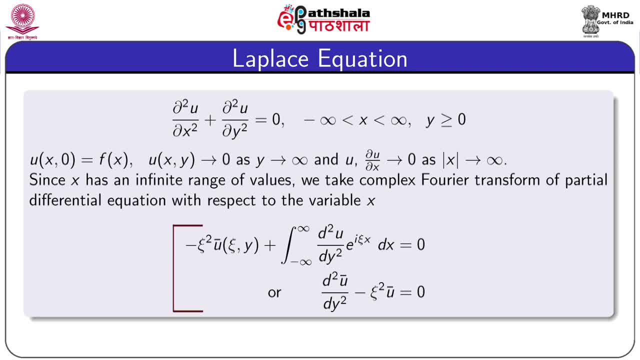 the expression which is given by the integration in this integral. if we interchange the differential and integral operator, then it gives d, 2, dy square of integration, minus infinity to plus infinity, u into e to the power, i, xi, x, dx. So that is nothing but u bar. So the second. 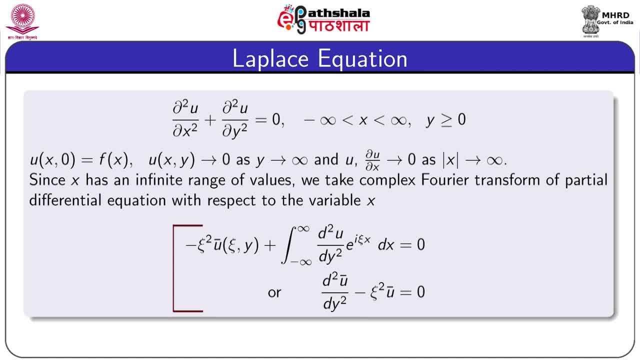 term in the expression is d 2 dy. So u bar d y square and the first term is minus xi square, u bar equals to 0.. Now this is the resultant equation. So this is an ordinary second order differential equation in u bar and the solution of this equation can be written easily. It is a into e to the. 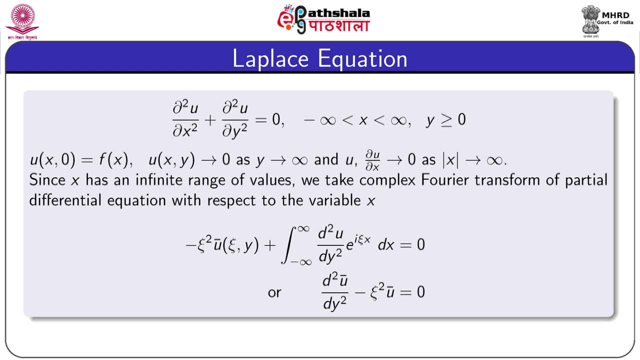 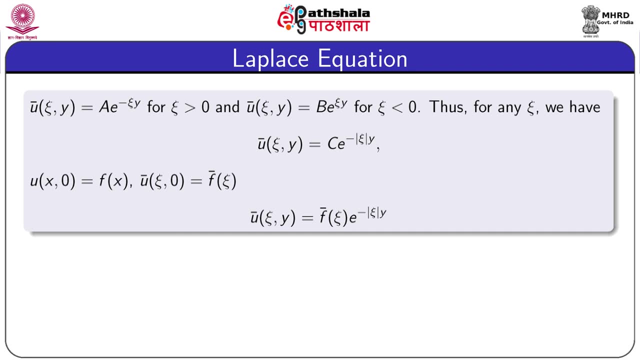 power xi into y plus b into d y. So this is the resultant equation. So this is an ordinary example. i i x, x explains in the earlier the same expression. i i x, x를 is upon the representation y sub i plus b into d y plus d y. So this is the Now to get the bounded. 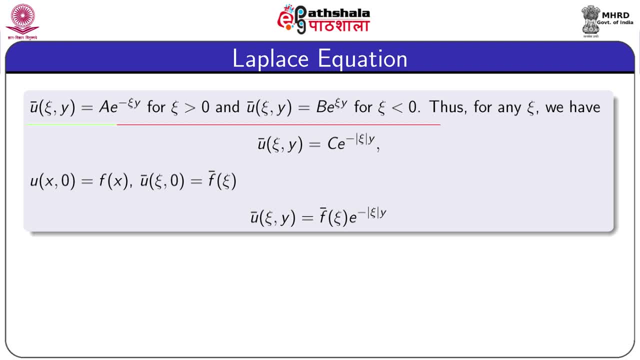 solution: u bar should have the functional form a into e to the power minus xi into y for xi greater than zero, and u bar equals to b into e to the power 0, step by step example. so this is an ordinary formula for this equation: u bar be into: 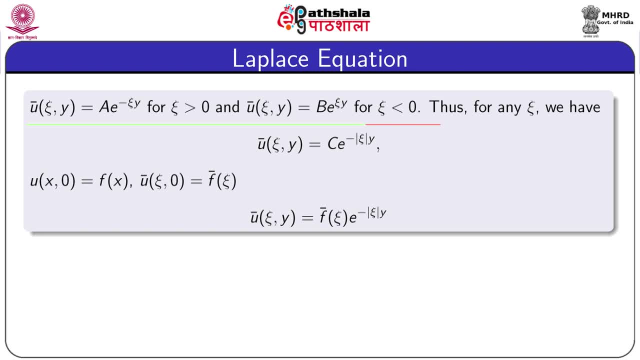 So here we consider sine for x, it becomes b, x, whole square, x x not the denken room, ou x y as 2. nota d n bar u bar is equal to b, e to the power minus xi, emperor, so E into the power xi, y for xi less than 0.. Thus for any xi, we can write the solution in the form: 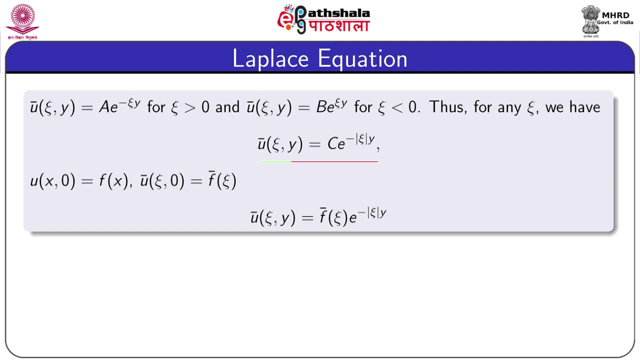 u bar is equal to c into e, to the power minus mod xi into y. Now to find the value of c we need to apply the initial condition. The initial condition is given: u x 0 is equal to f x. Now if we apply the Fourier transform of this equation, that gives u bar xi 0 is. 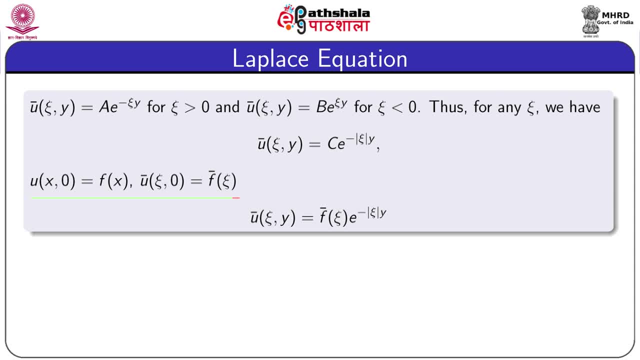 equal to some function: f bar xi. Now, if we use this condition to the solution, u bar equals to c to the power minus mod xi y. this gives the value of c is equals to f bar xi. Now, substituting the value of c in the general solution, our required: 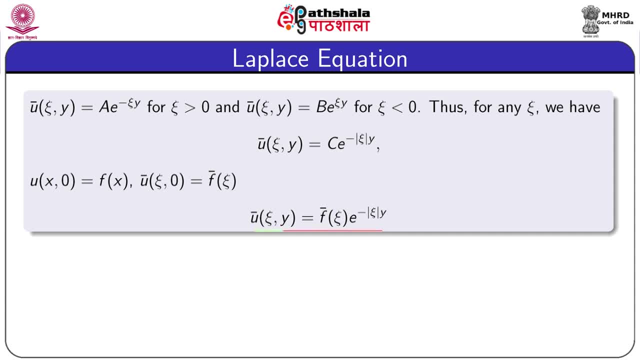 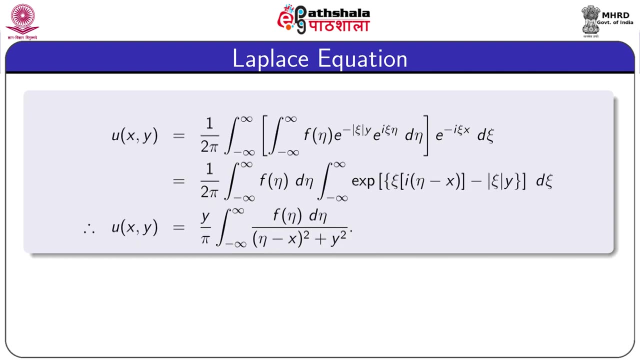 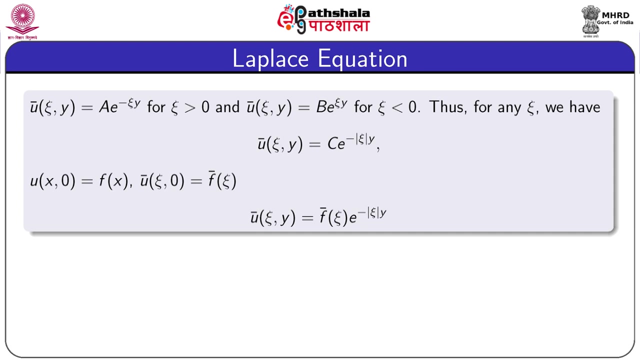 solution: u bar, which is function of xi and y, is equal to f bar xi into e, to the power minus mod xi into y. Now we have to find u as function of x and y. That means from this solution, in the expression for u bar we need to apply inverse Fourier transform to find u as function of x and y. 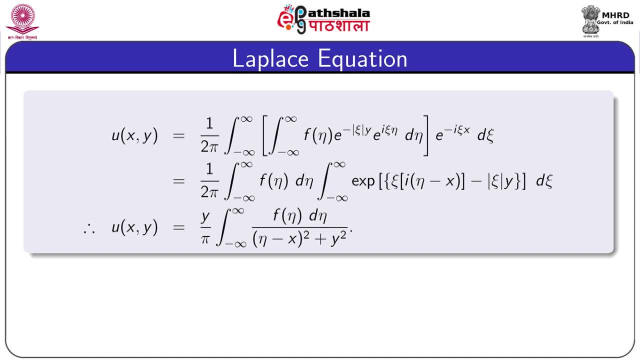 Now to obtain u as function of xi and y, we need to find u as function of xi and y. Now, to obtain u as function of xi and y, we need to apply inverse Flapler's transform of u bar. So the formula is written here: u is equal to 1 by 2 pi integration minus. 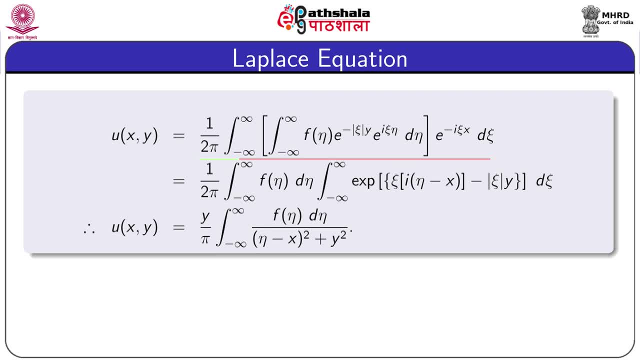 infinity to plus infinity, e to the power minus i xi x into f bar xi, And we have also substituted the value of F bar xi, which is written here, minus infinity to plus infinity, f eta, e to the power minus xi y e to the power i xi eta d eta this: 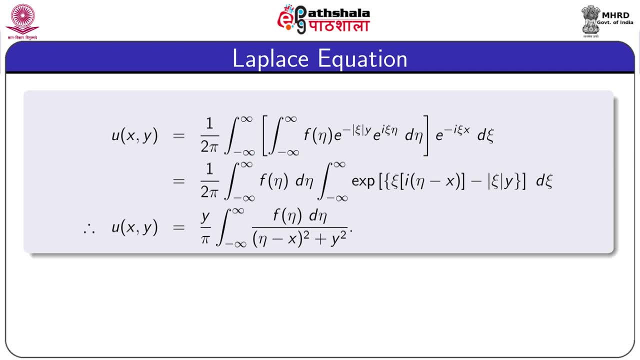 So in the next line this is equals to 1 by 2 pi minus infinity to plus infinity, F, eta, d eta. So we wrote the value of f up to here. So this accept the 제대로 integral at z x of: 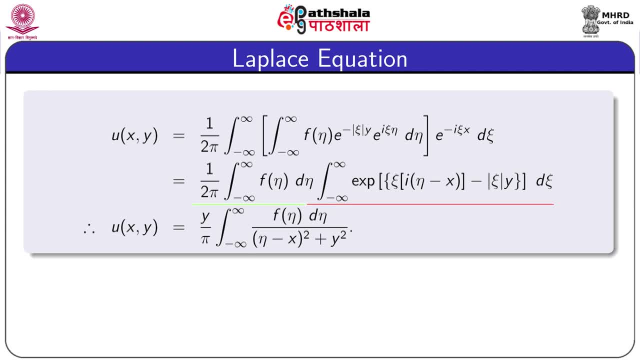 into integration, minus infinity to plus infinity, e to the power, xi into i eta, minus x, minus mod xi into y d xi. In the second line we interchange the order of integration. Now we can evaluate the second integral, and the value of the second integral is 1 divided. 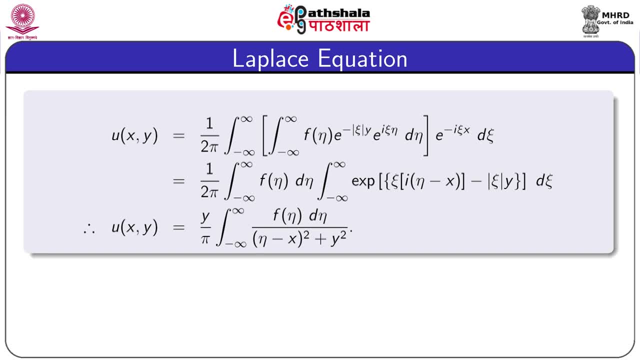 by eta minus x whole square plus y square. Therefore our required solution: u function of x and y is equal to y by pi integration minus infinity to plus infinity: f eta d eta by eta minus x whole square plus y square. Now we can evaluate the second integral, and the value of the second integral is 1 divided. 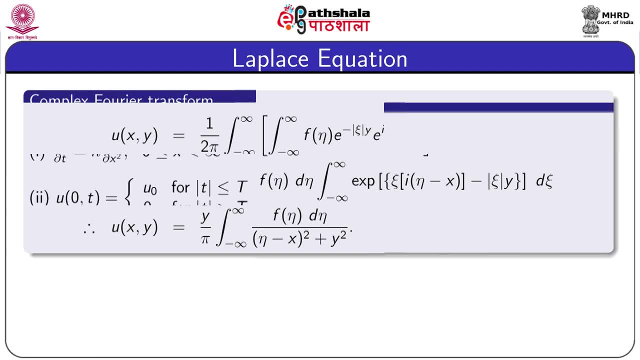 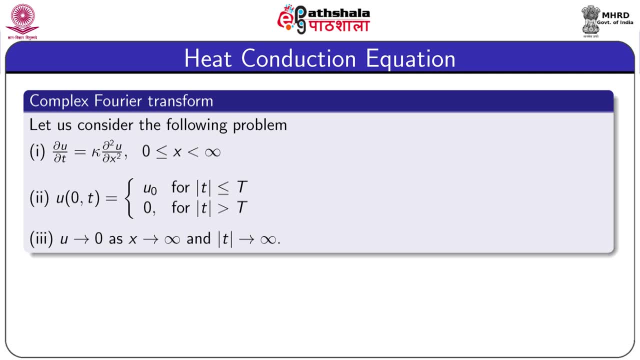 y square. Now we shall consider heat conduction equation and we shall apply complex Fourier transform to find solution of this equation. So the given equation is the heat equation, one dimensional heat equation in Cartesian coordinate system, which is given by equation one del u del t equals to kappa del t? u del x square, where 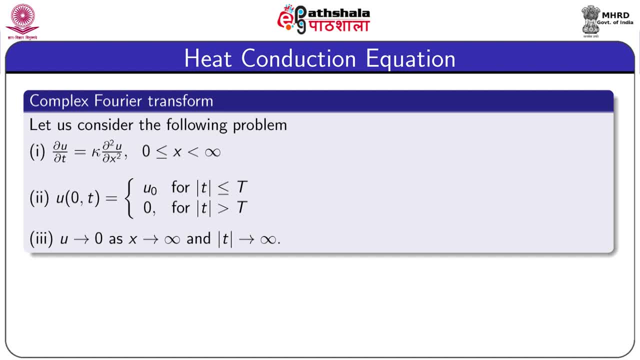 x lies between 0 to infinity and this equation is satisfied with the given condition. This is the boundary condition: u at x equals to 0, t equals to u 0 for mod t less than capital t and equals to 0 for mod t. 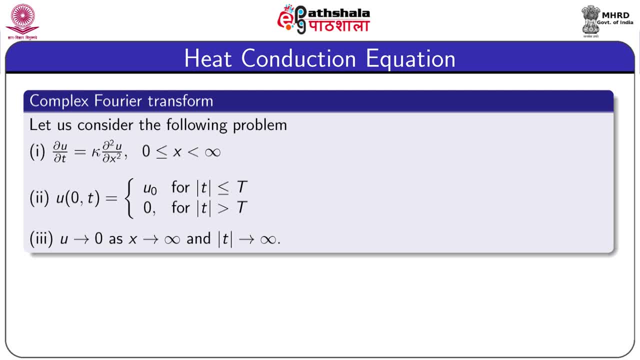 T greater than capital T and we also have: the solution is bounded. that means u tends to 0 as x going to infinity and mod t going to infinity. Thus we have to solve the conduction equation together with the condition which are given by 2 and 3.. 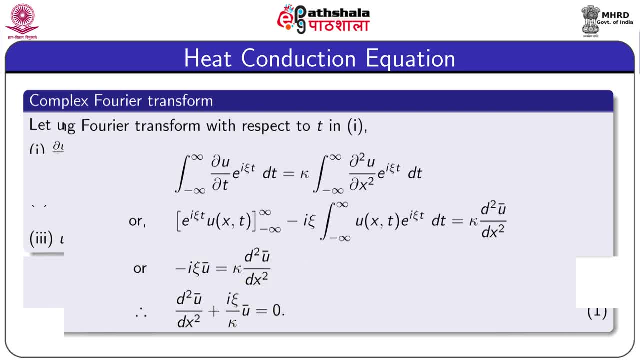 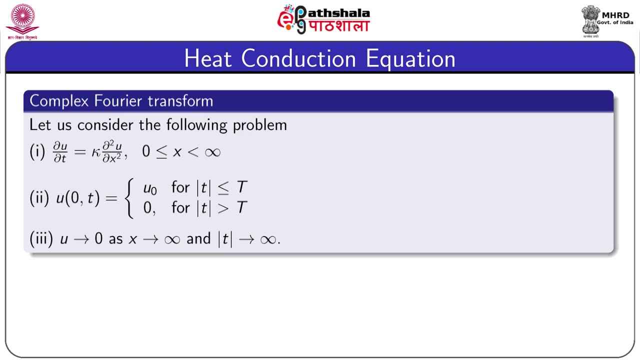 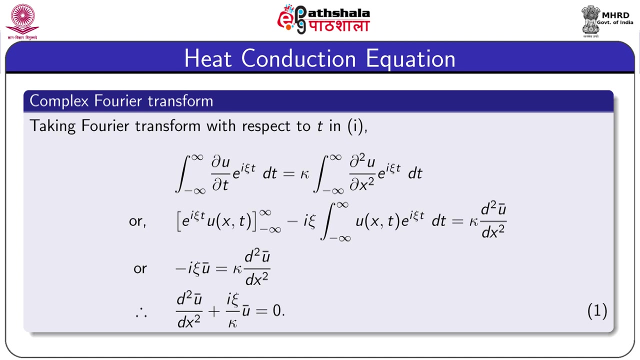 ão Fourier transform of u with respect to variable t and we have the condition that u tends to 0.. If you look back the condition 3, u tends to 0 as x tends to infinity and mod t tends. 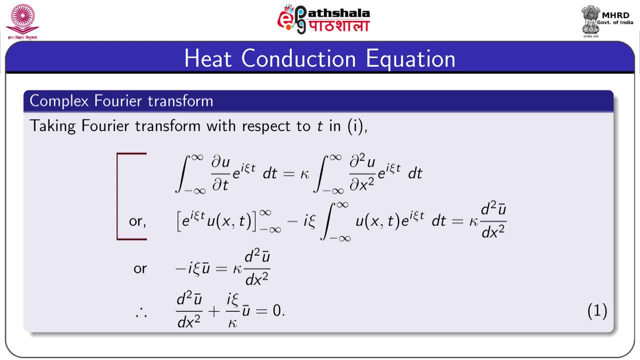 to infinity. So if you apply that, we get the term in the square bracket is 0. So this term is 0 and the second term is minus i. xi into this is nothing but Fourier transform of u with respect to t. For this problem we are denoting that by u bar, So left hand. 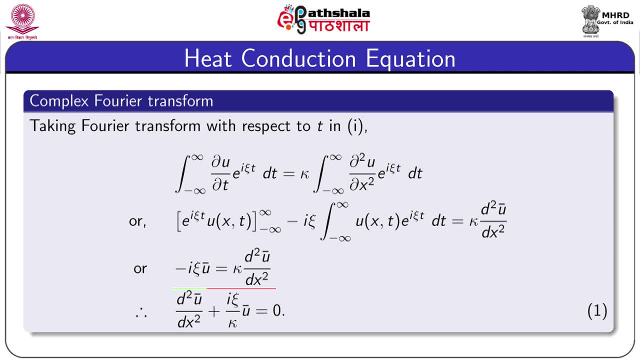 side is minus i xi u bar equals to kappa d 2 u bar d x square. So it can be written in this form also: d 2 u bar d x square, plus i xi by kappa u bar equals to 0.. Now this is a second order, ordinary. 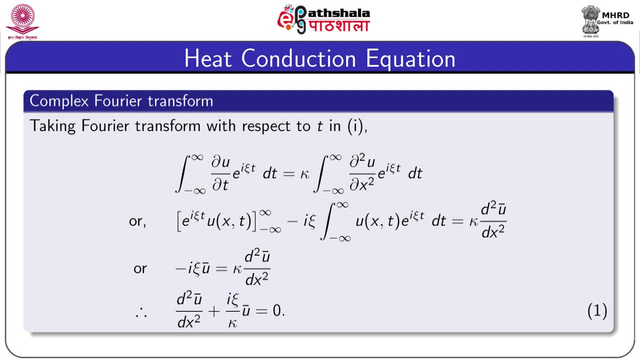 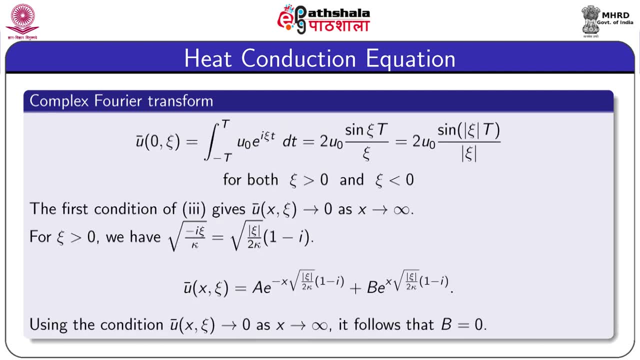 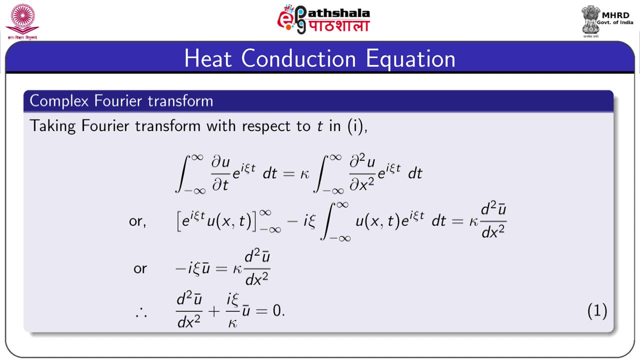 differential equation in x and the solution of this equation can be written in the form: u bar equals to a square root of i- xi by kappa into x plus b into e, to the power minus square root of i- xi by kappa into x, where a and b are arbitrary constants. Now we apply Fourier. 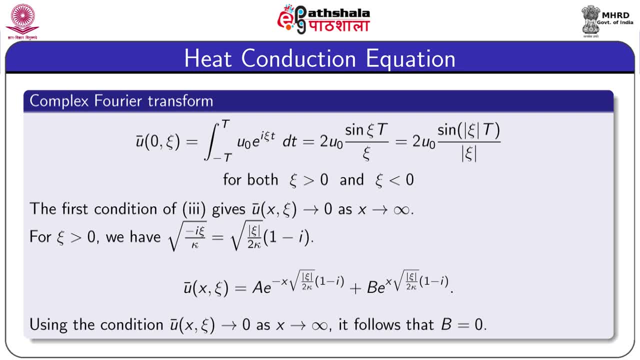 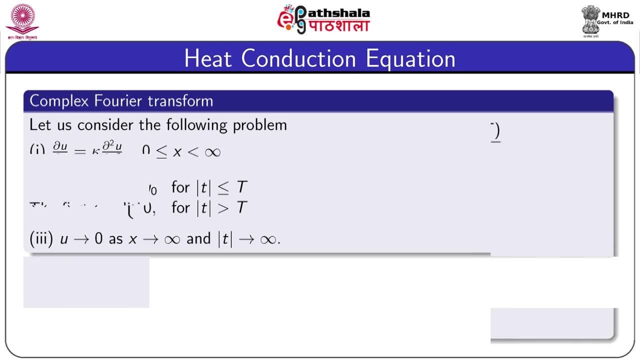 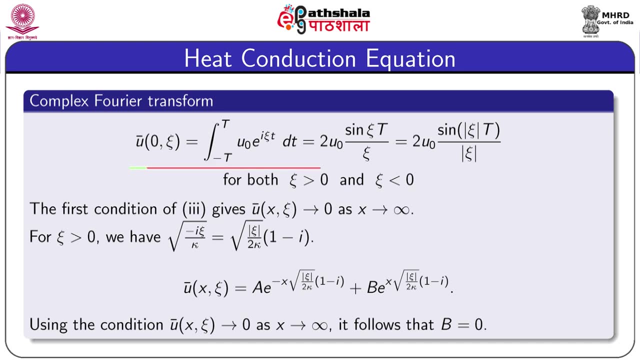 transform to the given condition. So if you look at this condition, condition 2,, this is the boundary condition. So if we apply Fourier transform to that, it gives u bar 0. xi is equal to integration minus infinity. to plus infinity, u 0 e to the power i xi. 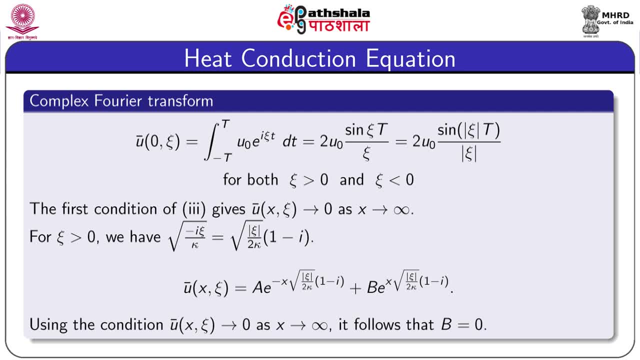 t, d, t. But we also have that the value of the Fourier of u is u, 0 within the interval minus t to plus t. So outside that interval the value of the integral becomes 0. So the limits of the integration becomes minus t to plus. 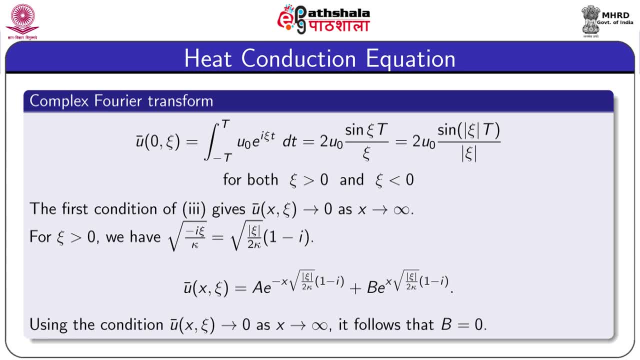 t. So after integration we get its value is equals to 2 u 0 sin xi t divided by xi. It can be written in the form also: So 2 u 0 sin mod xi t divided by mod xi, and these form is applicable for both xi, greater. 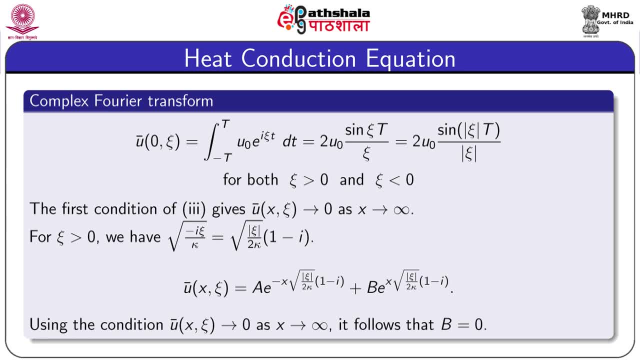 than 0 and xi less than 0.. Now if we look at the first condition of 3, which is: u goes to 0 as x goes to infinity. So in that condition, if we apply Fourier transform, we obtain u bar x. xi goes to 0 as. 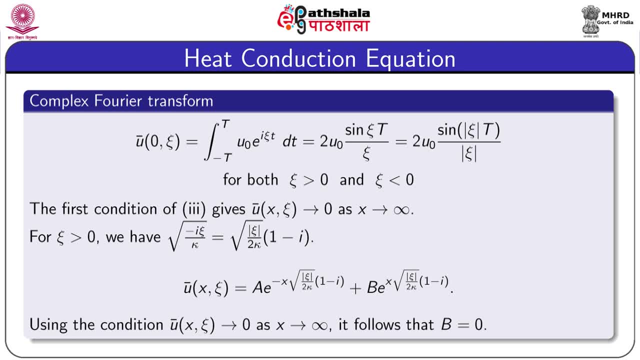 x goes to infinity. Now for xi greater than 0, we have square root of minus i xi by kappa e, square root of mod xi by 2 kappa into 1 minus i. So if we use that result, the general solution of equation one can be written in the form: u bar equals to A, e to the power. 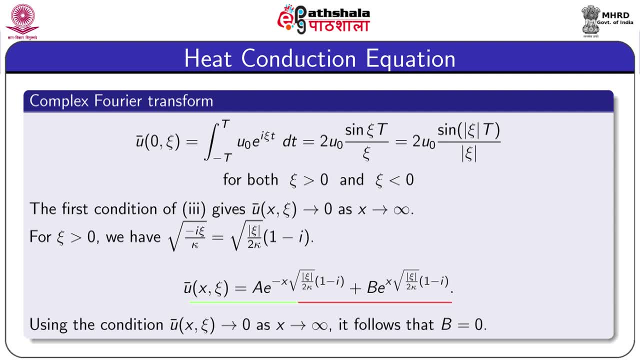 minus x square root mod xi by 2 kappa into 1 minus i. plus b bar equals to the power minus x Ohio. So this becomes a Aí ży by 2 kappa into 1 minus I. So if we use that result, the general solution of equation 1 can be written in the: 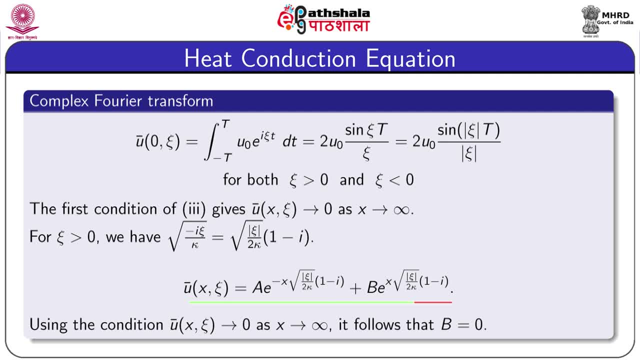 b e to the power x into square root mod psi by 2 kappa into 1 minus i. Now, using the condition u bar, xi tends to 0. as x tends to infinity, it follows that b is equal to 0. Because in this expression u bar, if b is there, then u bar will tend to infinity. 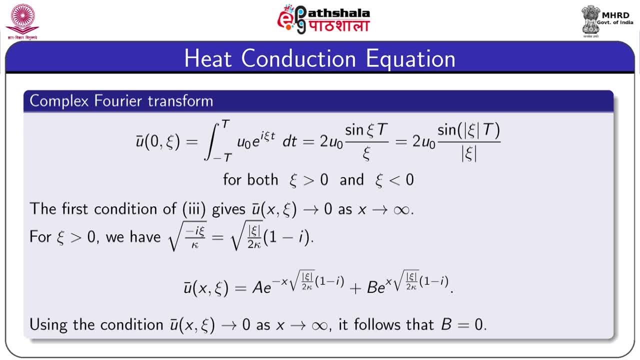 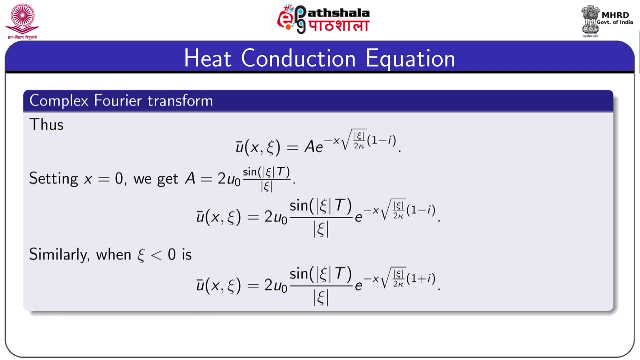 because the of this term, x, So b, cannot be a non-negative or non-zero number, So the only option is b is equal to 0. Therefore the general solution can be written as: u bar equals to a, e to the power minus x. square root mod psi. by 2 kappa into 1 minus i. 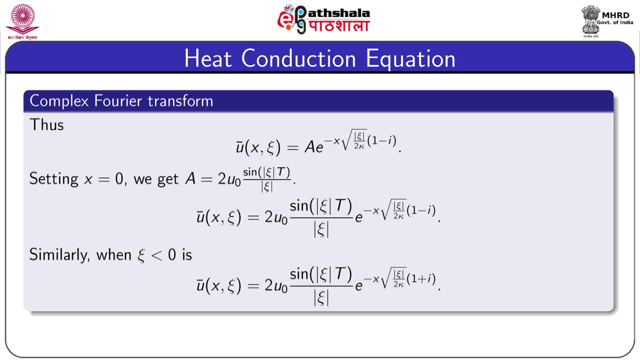 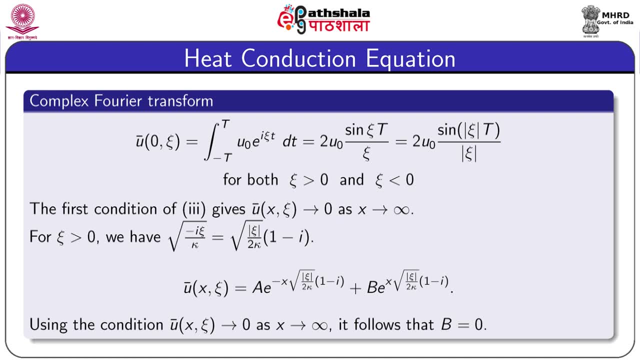 Now to obtain the solution. u bar xi tends to 0, as x tends to infinity. To obtain the value of a, we need to apply now the boundary condition: u bar 0, xi equals to 2 u 0 into sine mod xi, t divided by mod xi. If you apply this condition, this gives: 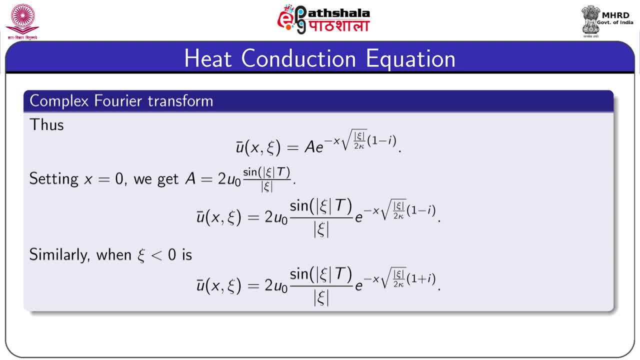 the value of capital A as 2 u 0 into sine mod xi t by mod xi. So substituting this value of a. Now our required solution becomes: u bar equals to 2 u 0 sine mod xi t by mod xi e to the power. 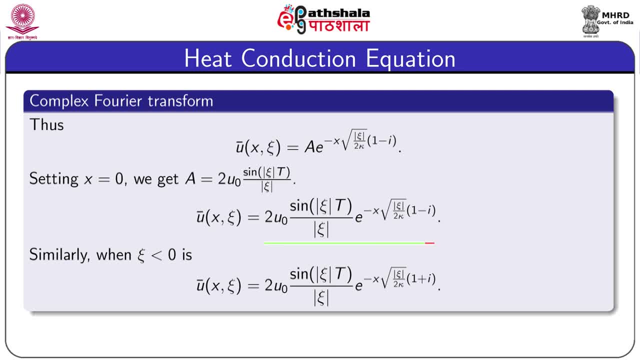 minus x square root mod xi by 2, kappa 1 minus i. So this is the solution for xi greater than 0.. Similarly, for xi less than 0, we can obtain the solution in the form: u bar equals to 2, u 0 into sine mod xi, t by mod xi e to the power minus x square root mod xi by 2. 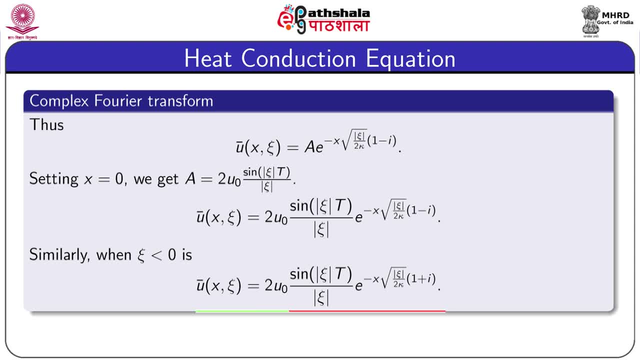 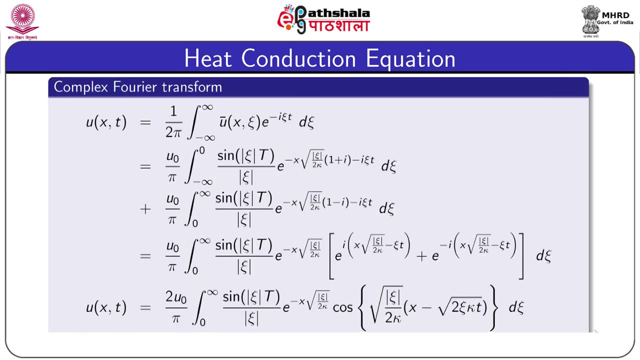 kappa into 1 plus i. Now to obtain u as function of x and t, we need to apply inverse Fourier transform. So this is the formula of inverse Fourier transform. So u x- t equals to 1 plus i. Now to obtain: 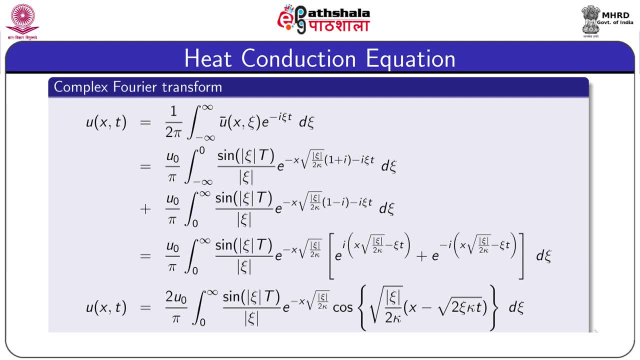 u bar equals to 2 u 0 sine. mod xi t by mod xi e to the power minus x. square root. mod xi t by mod xi e to the power minus i So u x t equals to 1 plus i So u x t equals to. 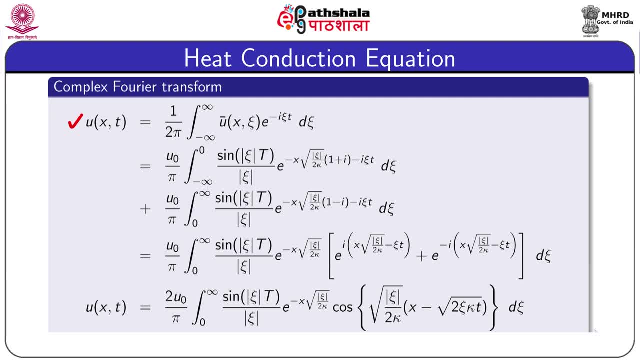 1 divided by 2, pi. integration minus infinity to plus infinity, u bar e to the power, minus i, xi, t into d, xi. Now we break the interval into two parts. One is for negative values of xi and the other is for positive values of xi. So in these two intervals we substitute: 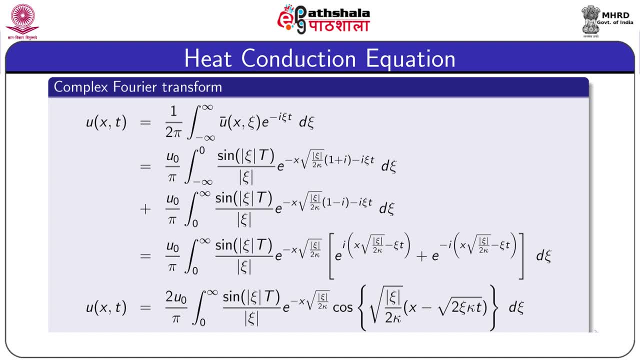 the values of u, bar and substituting these values, we obtain u as u 0 by pi. integration zero to infinity sine mod xi. t divided by mod xi. e to the power minus x. square root. mod xi by 2 kappa into e to the power i. x into square root mod xi by 2 kappa minus xi e to. the power minus x square root, mod xi by 2, kappa into e to the power i x square root, mod xi by 2. kappa minus xi divided by mod xi. e to the power minus x square root, mod xi by 2, und uniform nto you canPass boring and complete 0 by unionU to sulfur 같아. là여� ler can be terminated with. 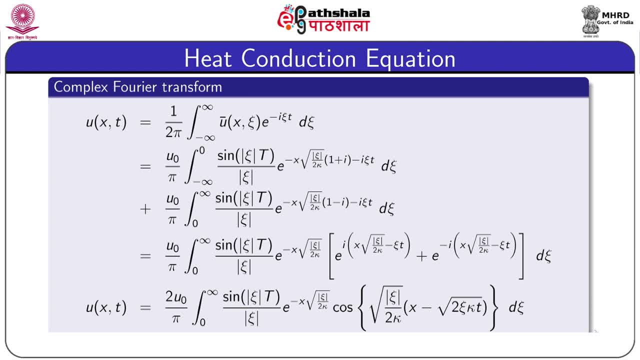 minus xi t plus e to the power minus i x into square root mod xi by 2 kappa minus xi t and this can be simplified to cosine function. So in the next line the term can be replaced by cosine function, which can be seen in this slide, the last line of this slide. So this: 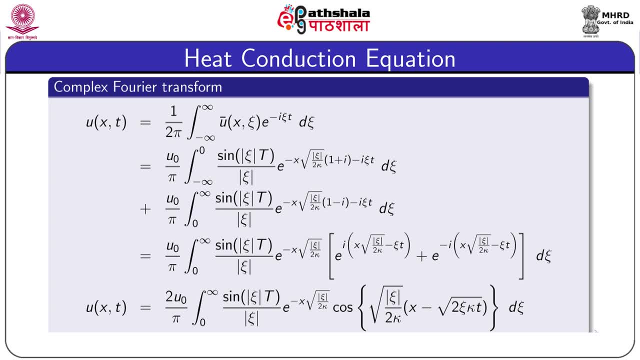 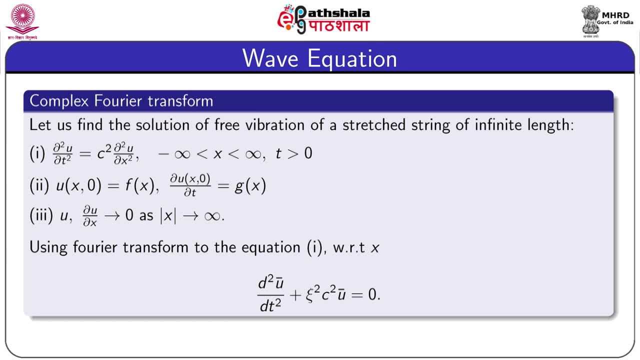 is our required solution. Now we are considering Fourier transform to find solution of wave equation. Now this is the equation: wave equation in Cartesian coordinate system, delta u, delta t square equals to C square. delta u, delta x square, where X has infinite proper from: 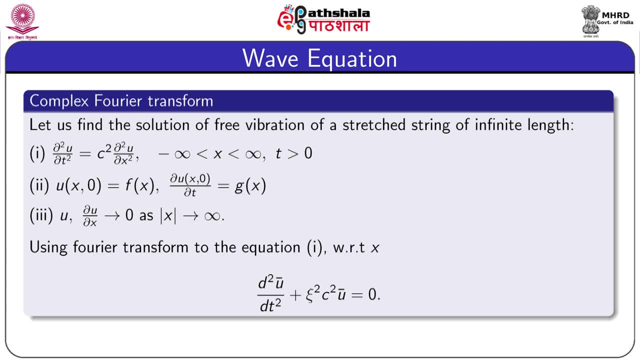 range and t is greater than 0, and we have also the initial condition: u at t equals to 0 is f x and del u del t at t equals to 0 is g x. and we also have u and del u del x tends to 0 as mod x tends to infinity. So first of all we take Fourier transform. 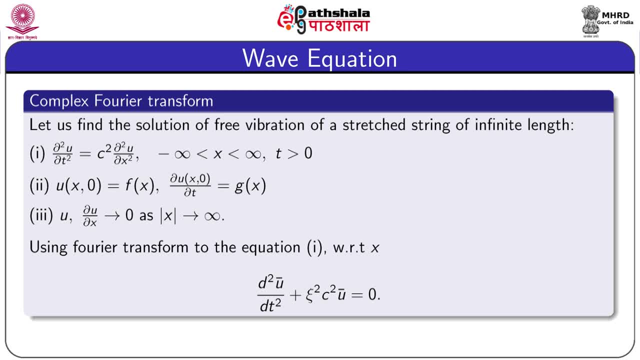 of the equation which is written in 1 with respect to x. So after taking Fourier transform, the equation becomes d: 2 u bar. d t square plus xi square c square, u bar equals to 0, where u bar is the Fourier transform of u with respect to x. 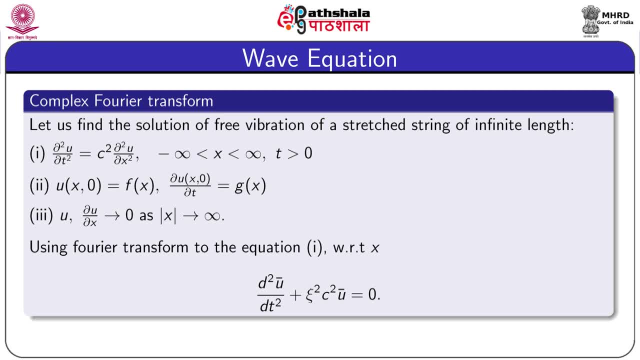 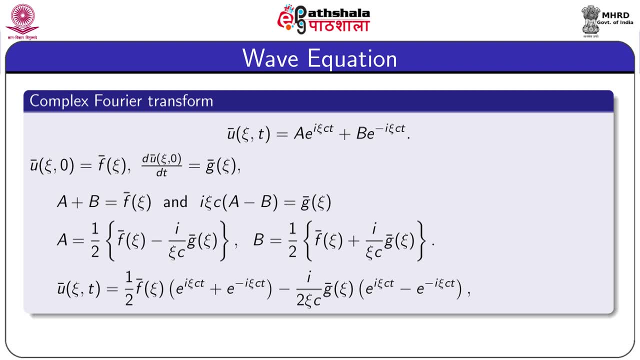 Now the solution of this ordinary differential equation is: u. bar equals to a, e to the power i xi c t plus b, e to the power minus i xi c t, where a, b are arbitrary constants. Now to obtain the values of these arbitrary constants, we need to apply: 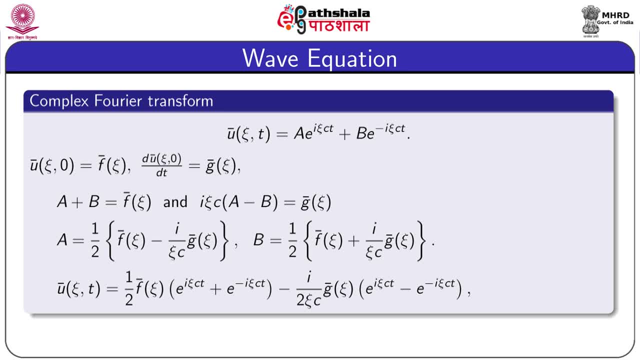 the initial conditions. The Fourier transform of the initial condition gives u bar xi 0 equals to f bar xi and d? u bar dt at point t equals to 0, is g bar xi. Now if we apply these two condition in the general solution, we obtain a plus b equals to f bar xi and i xi c into a minus b. 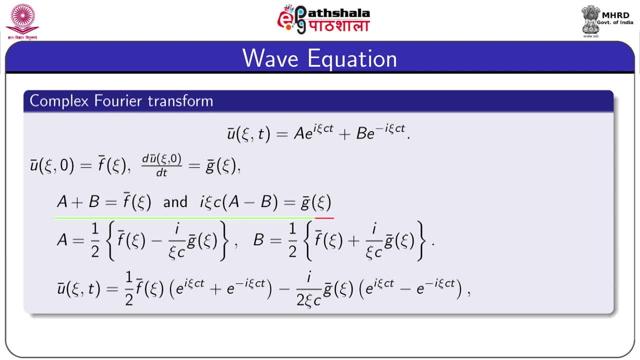 equals to g bar xi. So from these two equations we can obtain the values of a and b as a equals to half f bar minus i by xi, c, g bar, and b equals to a plus b equals to f bar xi. So from these two equations we obtain: a plus b equals to 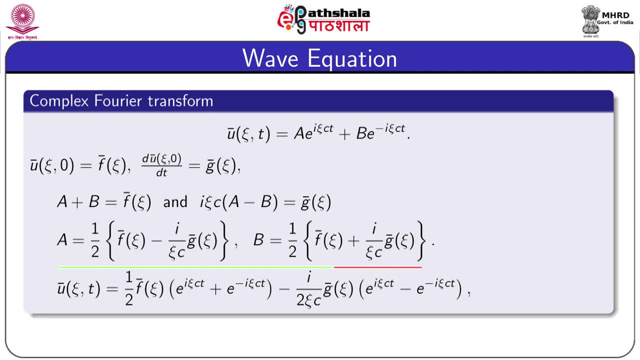 half f bar plus i by xi c g bar. So substituting the values of a and b in the general solution here we obtain u bar as half f bar into e to the power i xi c t plus e to the power minus i xi c t minus i by 2. xi c into g bar into e to the power i xi c t minus i by 2. 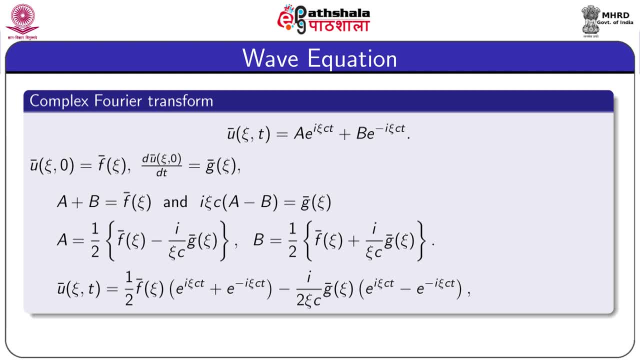 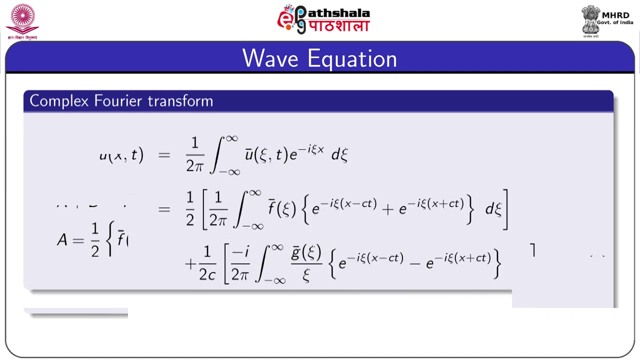 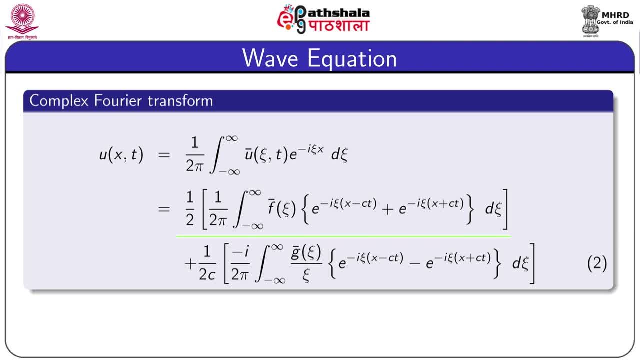 x plus ct dji plus 1 by 2 c minus i by 2 pi. integration minus infinity to plus infinity. g bar by xi into e to the power minus i xi. x minus ct minus e to the power minus i xi plus ct d j. 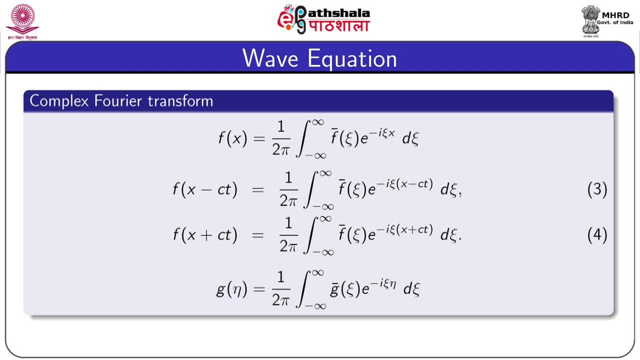 We know the expression for f x. this is the inverse Fourier transform of f bar xi. So f x equals to 1 by 2 pi integration minus infinity to plus infinity. f bar xi, e to the power, minus i, xi, x, d, xi. So in this expression, if you take the argument of f as x minus c, 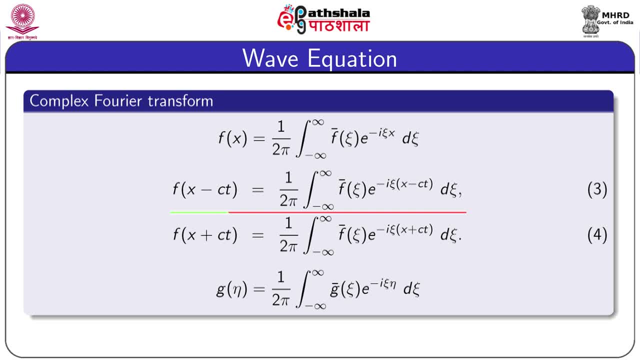 t. So value of f x minus c t is equals to 1 by 2 pi minus infinity to plus infinity, f bar e to the power minus xi into x minus c t. So x will be replaced by x minus c t in this expression. Similarly, the value of f? x plus c t can be: 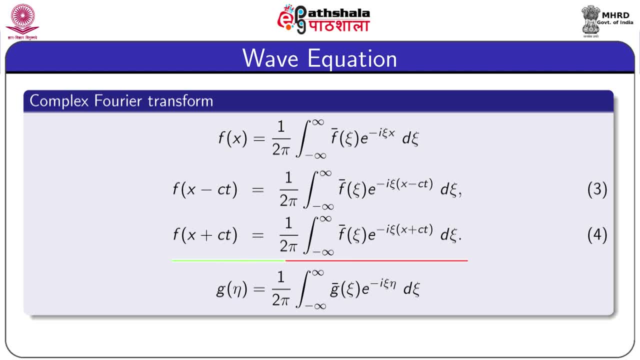 obtained from the expression of f x by replacing x by x plus c t. So the expression for x plus c t is given here. and we also have g eta. this is inverse Fourier transform of g bar. So g eta is equals to 1 by 2 pi minus infinity to plus. 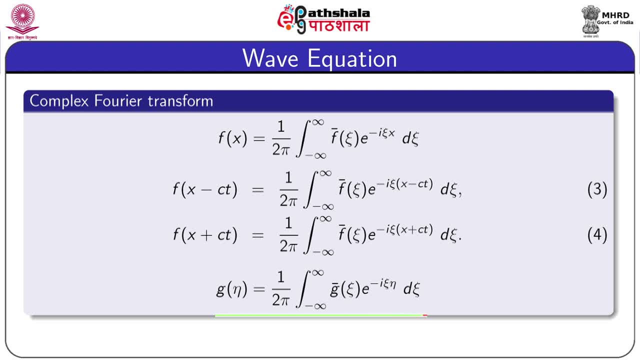 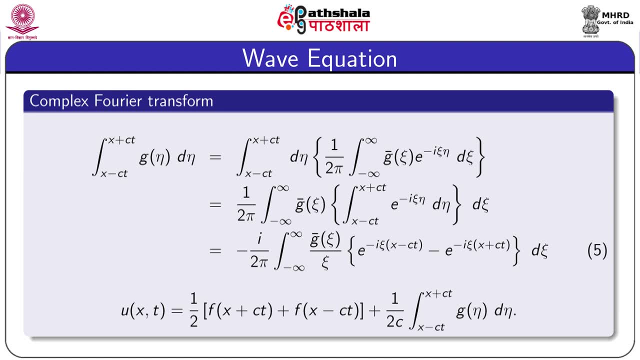 infinity g, bar xi, e to the power minus i, xi, eta, d, xi, And in this expression you can see that integration x minus c t to x plus c, t, g, eta, d eta is equals to integration x minus c t to x plus c, t, d eta, and this is the expression for g eta. 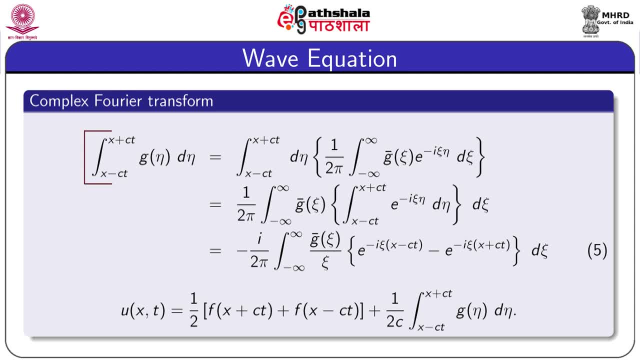 So this equals to 1 by 2 pi. minus infinity to plus infinity, g bar g, eta e to the power, minus i, xi, eta d xi. So this equals to 1 by 2 pi. now we interchange the order of integration, So it is minus infinity to plus infinity, g bar xi and this: 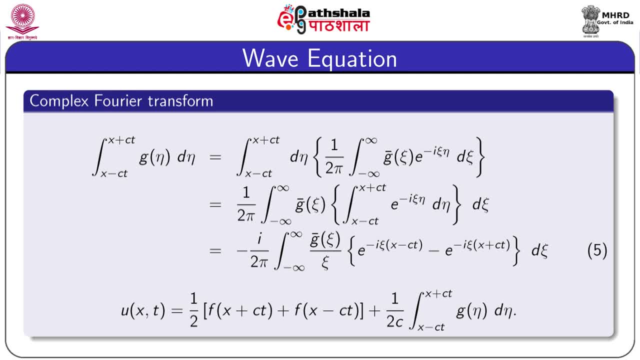 is x minus c, t to x plus c, t, e to the power minus i, xi, eta, d, eta into d, xi, And we can find the value of this integral. And value of this integral becomes here, which is written here: e to the power minus.